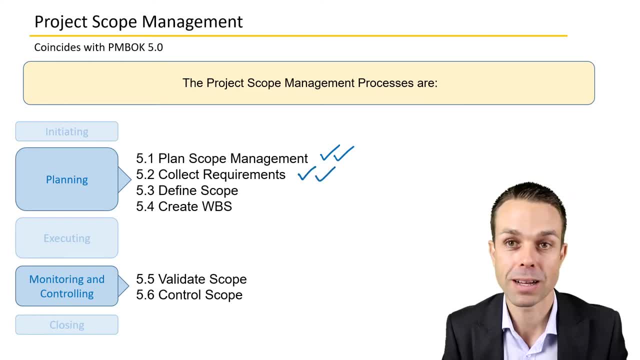 the overall approach. then we're collecting the requirements from our customer or whoever we're delivering the project to. then we're defining the scope from those requirements. then we're creating the work breakdown structure. So, from the scope, what are the activities that we need? 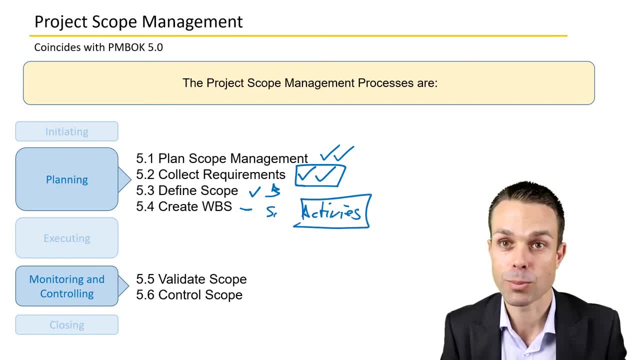 to do to make that scope happen and actually create the project and create the project deliverables. Then, once we've delivered them, as you can see, we've got the scope management processes where there's nothing in executing. So executing the project work happens outside of this knowledge. 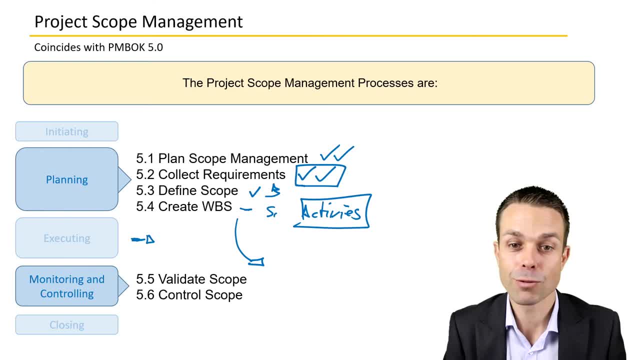 group. but once we have executed all of those deliverables, we need to validate that scope. So the customer needs to say, yes, this is the right specifications and they're accepting those deliverables. And then we also need to control scope. So we need to make 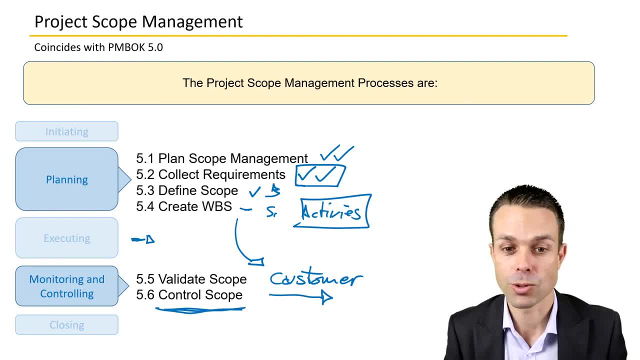 sure that it stays on track. Is it what we wanted to deliver? Does it need to change? If it needs to change, we might need a change request, as noted in our change management plan, And so those are all the processes as part of project scope management. There are a lot of inputs. 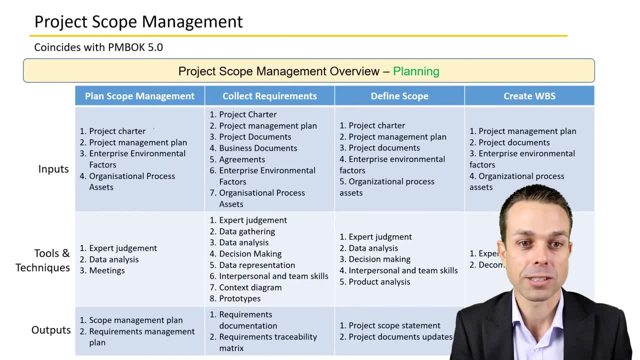 tools and techniques and outputs that you'll see as well. The project charter comes up a lot for all of these particular ones And of course the project management plan is an input into all of these processes as well. You'll also see a lot of enterprise, environmental factors and organizational 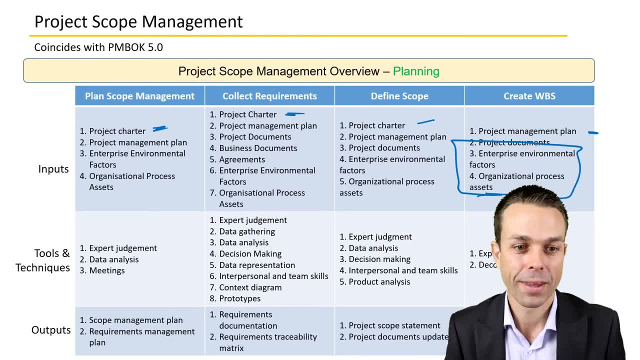 process, assets as an input And, of course, expert judgment. you'll see a lot of as well. Look at all of those for all of the processes there. You'll also see decision making, a lot of decision making, And decomposition is one of those things that we need for the work breakdown structure where 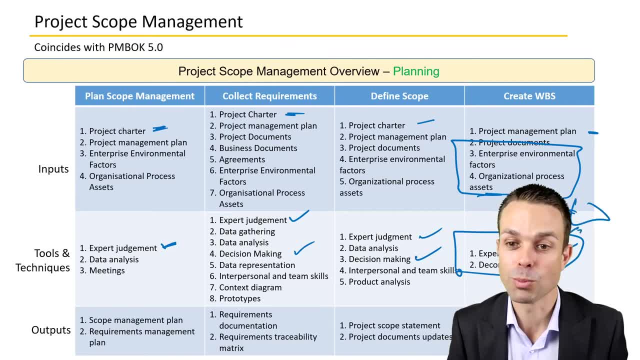 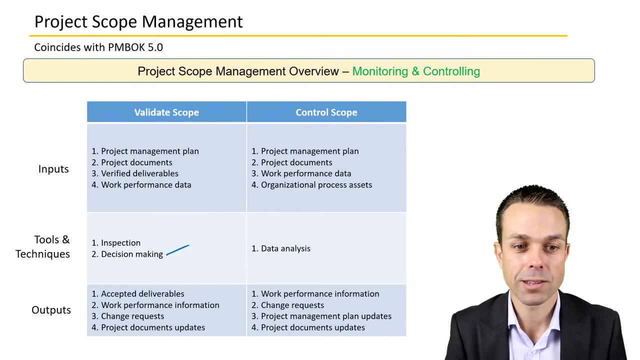 we're decomposing large features into smaller and smaller parts or activities that we can actually perform. You'll see decision making come up again- And, of course, things like inspection. We're inspecting those deliverables and making sure that they are as we wanted them to be, and some 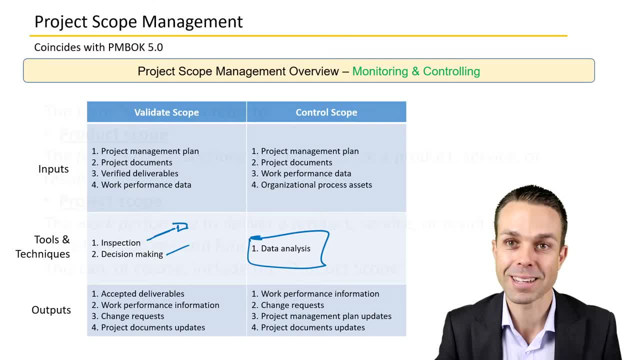 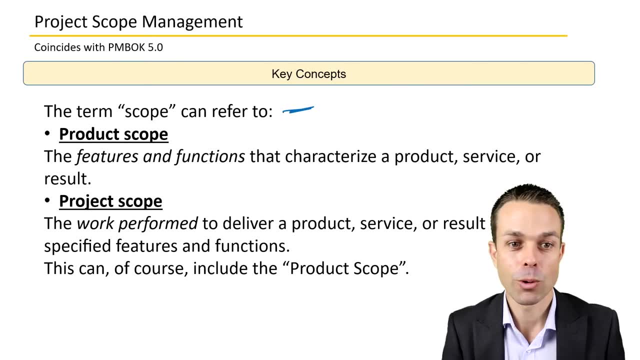 data analysis as well, to make sure that we are on track. Key concepts for project scope management. We've got the term scope. This can refer to two things. We've got the product scope. This is the features and functions that characterize a product service. 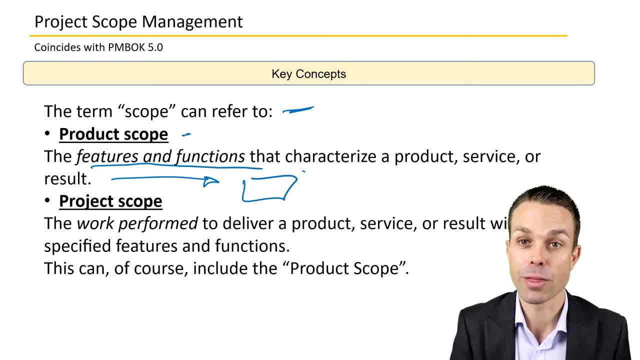 or result, Typically what we are delivering: the product. So what is the scope of the product? Now we can also have the project scope scope: this is the work that we're performing to deliver that product, that product, service or result and the specified features and functions. so this 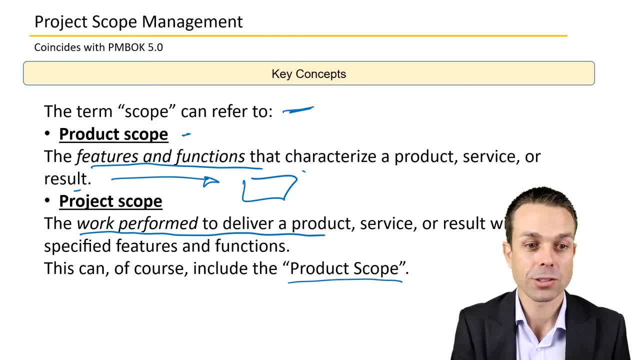 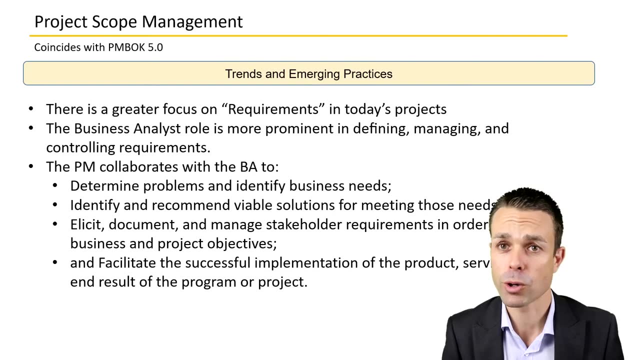 can, of course, include the product scope. so project scope is: is the work performed? so what work are we doing? but the product itself is: what are we delivering? trends and emerging practices in project scope management. there is a greater focus on requirements in today's projects, specifically with the rise of 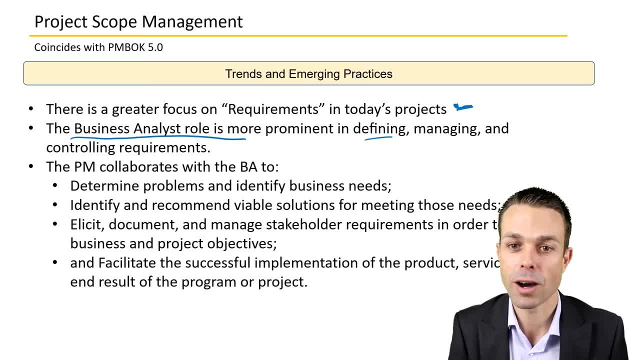 the business analyst role, so it's more prominent in defining, managing and controlling those requirements as you go along in your project. that means as a project manager you'll probably have to work with a business analyst to determine problems- the original problem that you're trying to fix and identify. 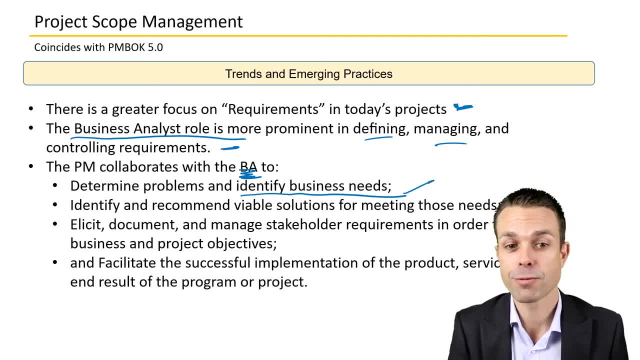 those business needs. so gathering those requirements, identify and recommend viable solutions for meeting those needs. and then a little bit of a summary of what we're doing today is we're going to focus on the next steps. what is a business analyst dese or a projectes, sk Sasha. 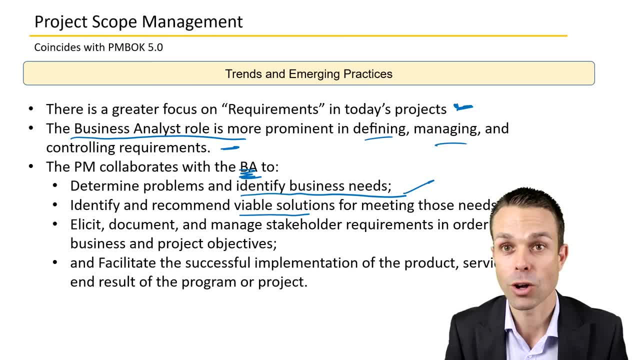 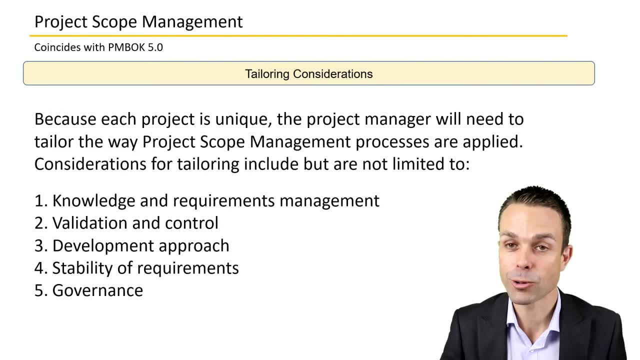 and, of course, the toast board that our team will be presenting. and then, of course, I've given it about a thread and in the chat box, please think of the characteristics of the project together. so the principles are as instruments of a project. so in the first step we will be looking at whether you are doing. 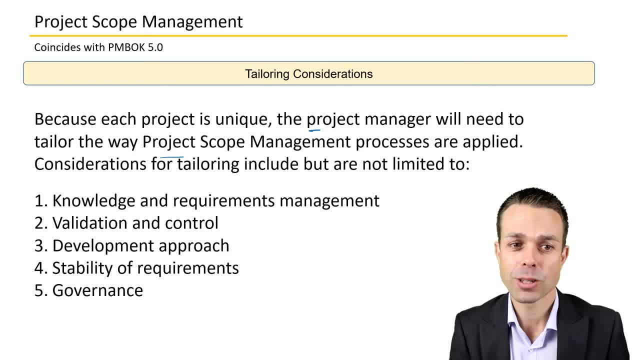 staff Superintendent, Have you worked a step in by yourself? have you done a? tailoring might include the validation or control aspects, The development approach. So how are we actually going to work as a project? Is it a waterfall method? Is it an agile method? The 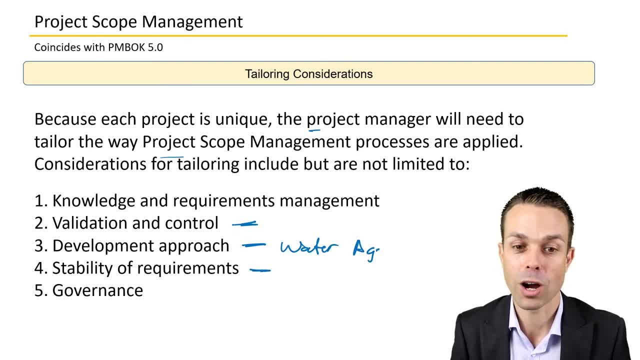 stability of the requirements. Now that's a big one. Are the requirements subject to change? Do we know if they're going to change a lot, or do we have an indication of that? Maybe, if it is going to change a lot, it's better to use an agile approach, which is much better in the face of